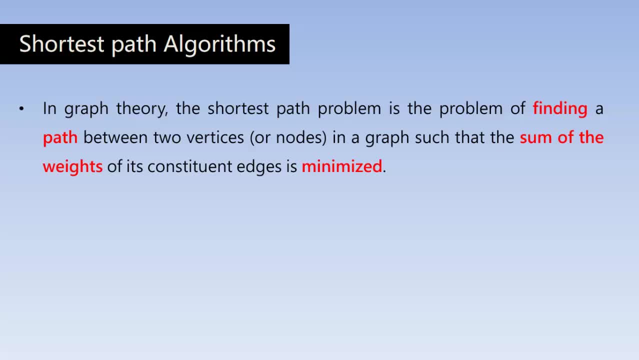 reach that place. So you are going to find that and you will go on that way To solve the shortest path problem. we have so many algorithms and in the series we will be learning the three important and popular algorithms. that is, the Disgrass algorithm. 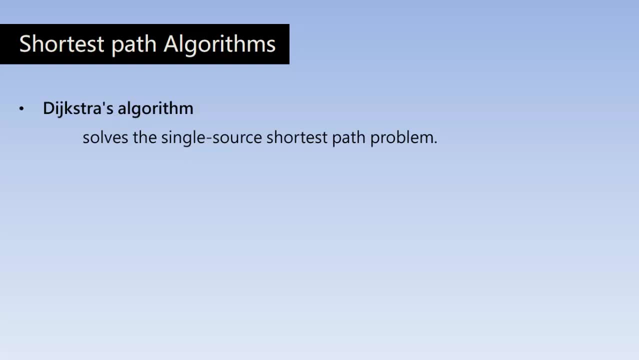 It solves the single source shortest path problem. That means we are given a graph and we are going to find the shortest path from a source node to all the other nodes that are in the graph. So this is called the single source shortest path problem. 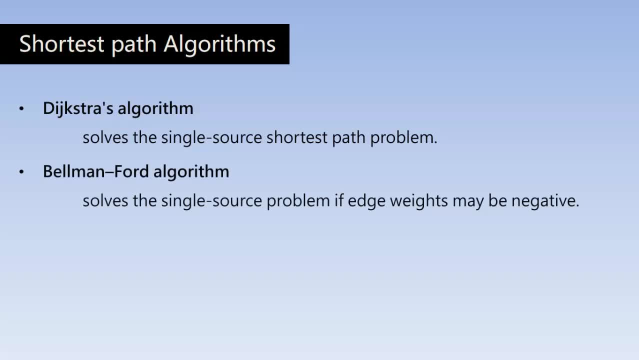 And the other one is Bellman-Ford algorithm, which solves the single source problem even if the edge weights are negative. Normally when we are solving the shortest path problems, weight should be given there for every edge. If the edge is given the positive weight only, we can solve that using Disgrass algorithm. 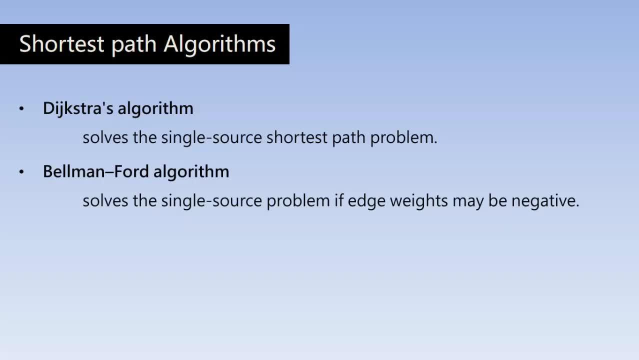 If you are given the negative weights, you can go for Bellman-Ford algorithm. And the last one is Floyd-Warshall algorithm, Which solves all pairs: shortest paths. This means here in this algorithm, we are going to find the shortest path between every. 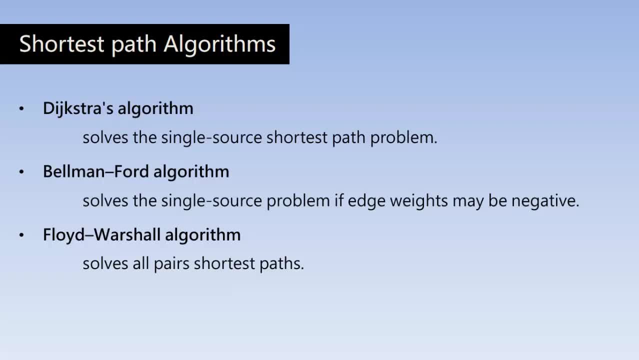 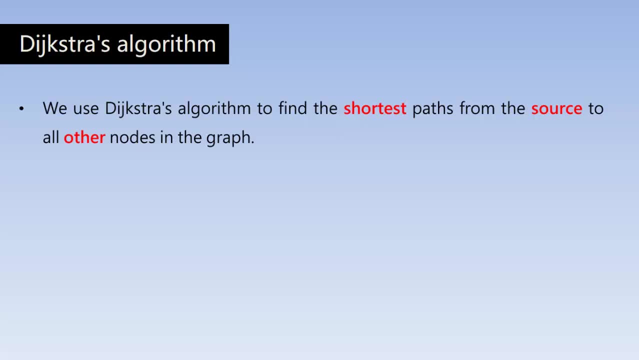 pair of nodes in the graph. In today's video we are going to learn the Disgrass algorithm. We use Disgrass algorithm to find the shortest paths from the source node to all the other nodes in the graph. For a given source node in the graph, the algorithm finds the shortest path between: 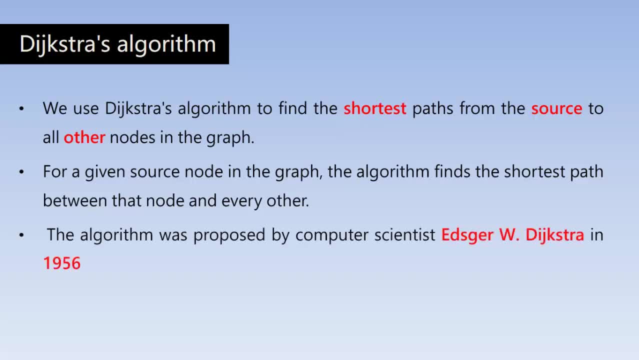 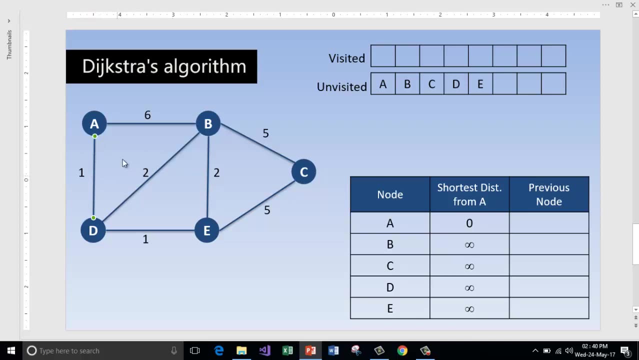 that node. So we are going to find the shortest path between every other node, And this was proposed by a computer scientist called Edgar W Disgrass in 1956. So let's go and do that. So here is the graph, and every edge between the nodes have the weights. 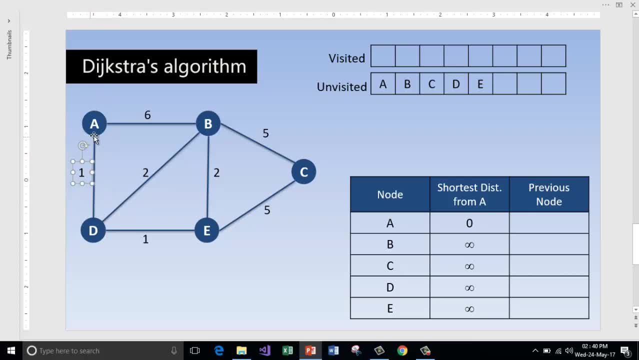 So to reach from A to D, it takes one unit, and to reach to B from A, it takes six units, and so on. Here we are going to make use of two lists: One is for storing the nodes which are visited, and the other one is for storing the nodes. 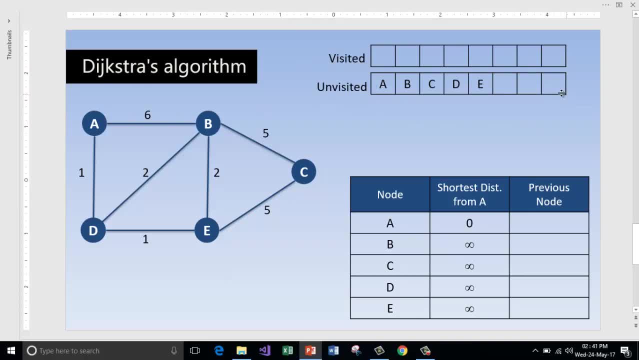 which are unvisited. Currently we have not started the algorithm, so all the nodes are unvisited And the table where we have got the list of nodes in the first column and the shortest distance from the source node- In this case A A- is the source node. 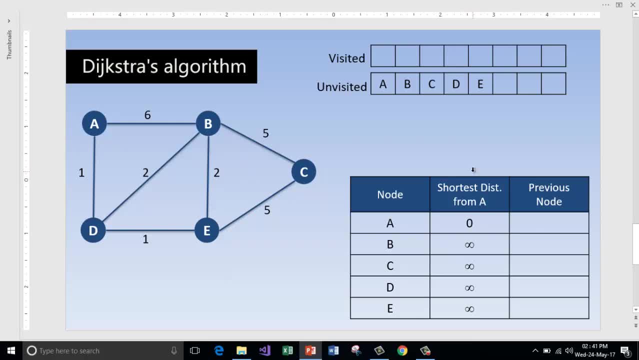 And in the second column we are going to store the shortest distance from A to all the other nodes, And in this third column we will also keep track of the previous nodes via which we get the shortest node to reach this node. So we are going to do that. 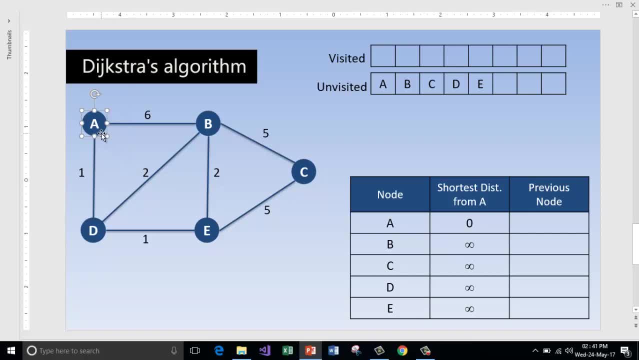 So, starting from A now, A is our starting point, So to reach A from itself, it takes zero cost. That is why it is initialized with zero And we have not yet started the algorithm To reach all the other nodes, from A to D, it takes zero cost. 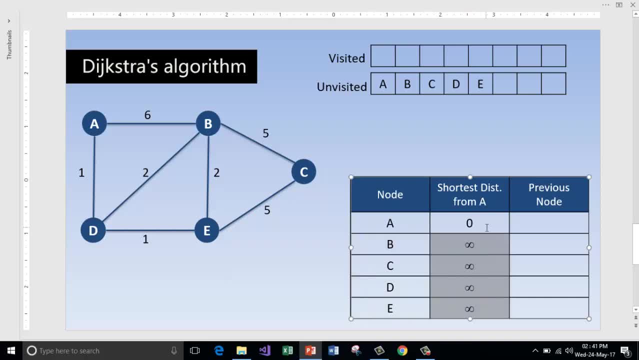 So we have not yet started the algorithm. To reach all the other nodes, from A to D, it takes zero cost. So to reach all the other nodes from A is infinity, because the value is not calculated yet. so we have initialized with infinity. 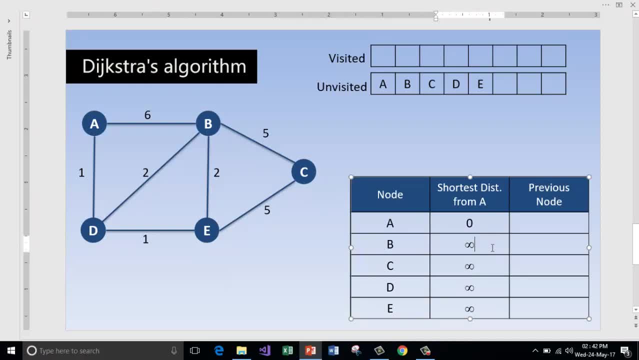 Once we calculate, we will erase this all and replace with the value calculated. So let's start from A. Now unvisited nodes which are reachable from A. The nodes D and B are the only two nodes which can be reachable from A and which are unvisited. 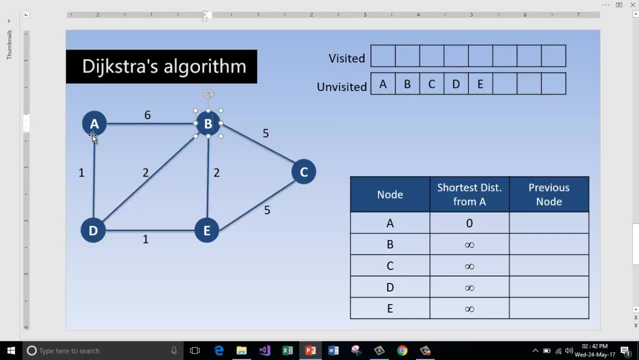 So D takes 1 and B takes 6. 6 to reach from A Right. So here we are going to write that information in this table: To reach B it takes 6 units. To reach D it takes 1 unit Right. And the previous node: 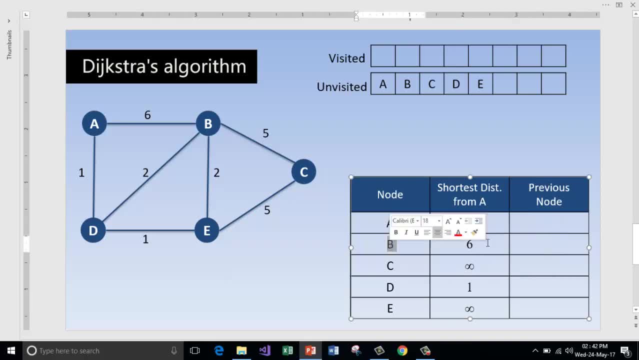 to reach B via which we got to B is A, And here also it is A Right. So now A is visited, So this is no longer be touched at all. So I will mark this as visited by some color. 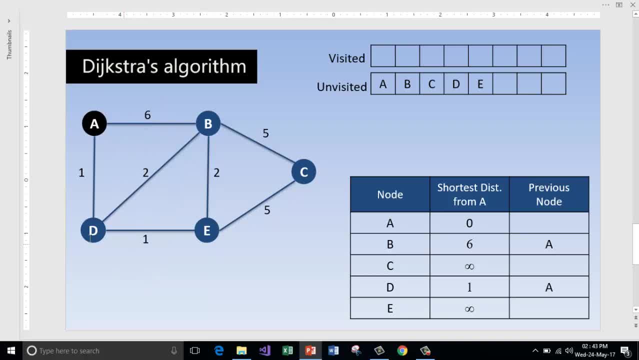 say black Right. So now visit that node which has got the minimum cost from the starting node. So B has got 6, but D has got just 1.. So now I visited D, Right Now identify. 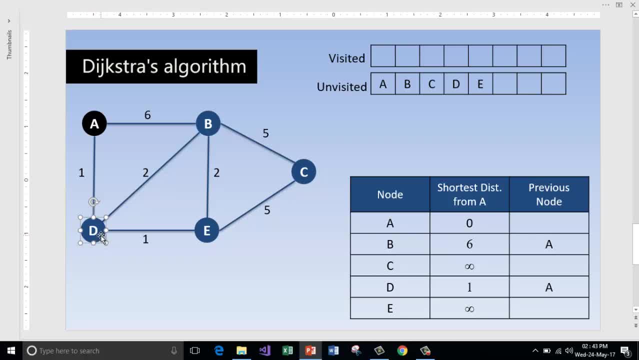 those nodes which are reachable from D which are not visited, That is B and E. Now go and update the information in the table for the shortest distance from D Right. So for B, the minimum cost to reach to B is 6 earlier, But now it is 3.. So how it is 3?? Because 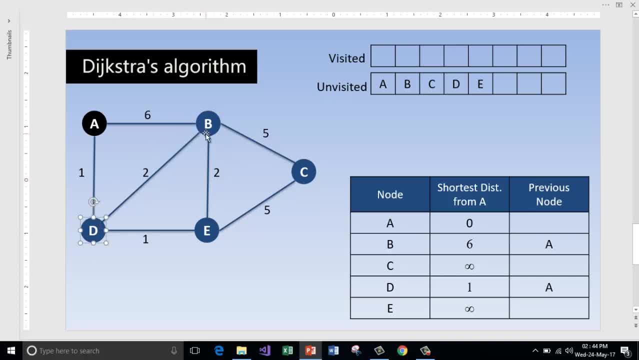 now we are reaching B via D, So the cost involved to reach B is 1 plus 3.. So now we have got the new minimum cost, which is much lesser than the earlier. So now it is the time to update. 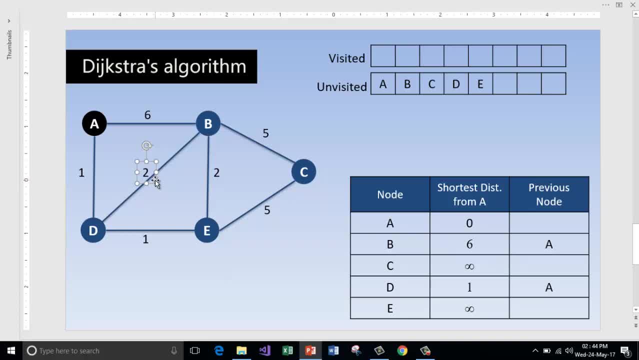 Whenever we get the new cost from B, we are going to update D from the beginning But cost, which is minimum and you are finding the earlier cost is maximum. just replace that Now to reach B. it is just 3 units and the previous node is D. Now to reach. 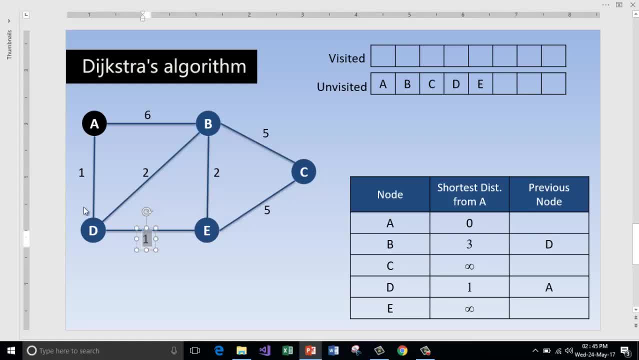 E, it takes just 2 units. Why 2 units? Because one from A to D and another one from D to E. So to reach E it takes 2 units. So now I will erase this infinity and I will enter. 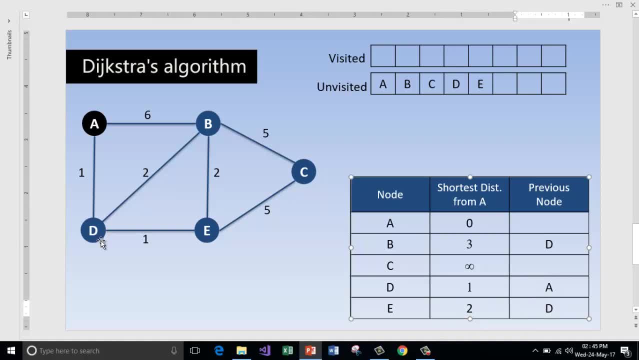 2. And the previous node is D. Now I visited D and I will mark it as visited. That's right Now, from D. now we are going to visit that node which has got the lowest cost from the starting node, that is E, because it has got just 2 units. 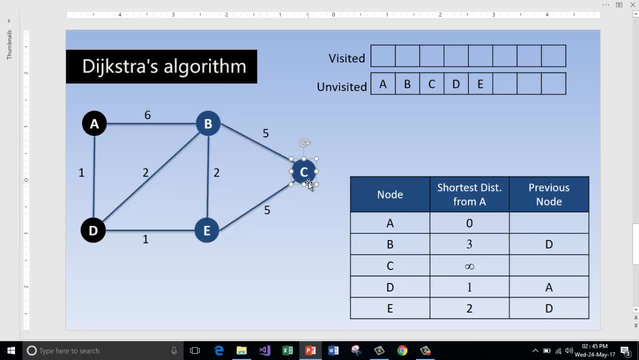 Now From E, B and C are reachable and those two are also not visited. Now we are going to calculate the cost involved in reaching B via E and same with C via E. The cost involved in reaching B is 1 plus 1 plus 2, 4.. 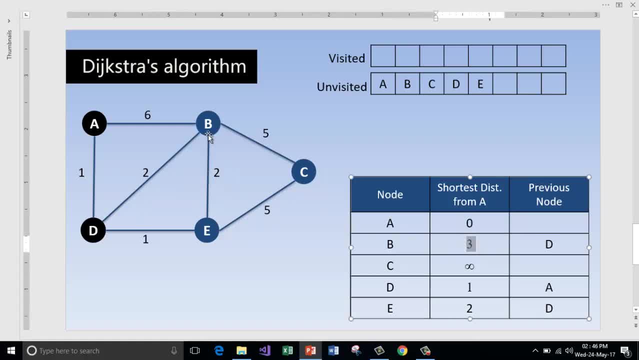 So now it is 4 to reach B. Earlier it was 3.. The newly calculated cost is higher than the earlier, so we are not going to disturb this cost because this is lesser, even lesser. Now. the cost involved in reaching C via E is 1 plus 1 plus 5, which is 7.. 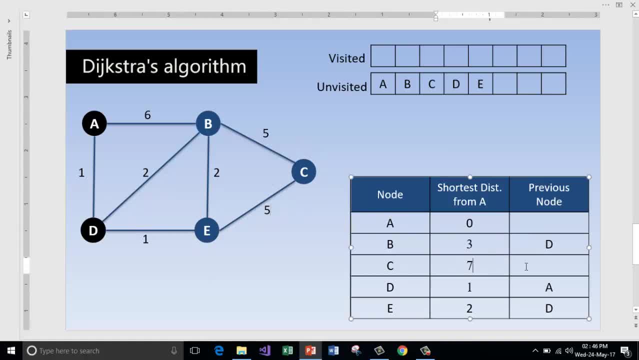 Earlier cost was infinity. so we will replace this and we will update the previous node as E, because via E I have got into the node C. So now this is over, Let me mark this as visited. Now go to that node after E which takes the lowest cost. 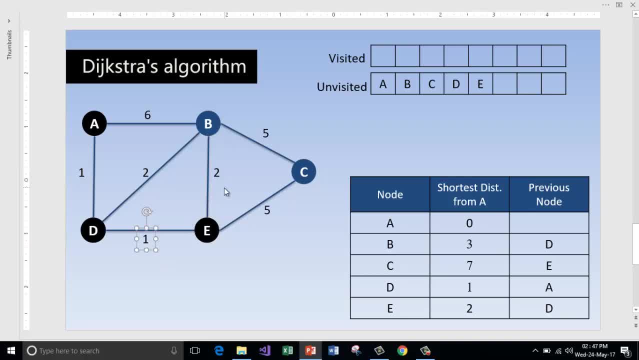 So to reach B, it takes 1 plus 1 plus 2, 4.. To reach C, it takes 7.. So 4 is the minimum cost. so now I will go and visit the B. So now, from B, the only node that can be reachable is C. So let's go and find out the distance. 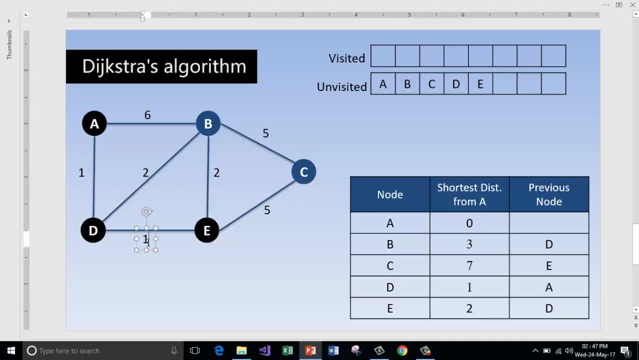 to C: 1 plus 1 equals 2,, 2 plus 2 equals 4,, 4 plus 5 equals 9.. To reach C it takes 9 units via B, E and D, but earlier cost was 7.. 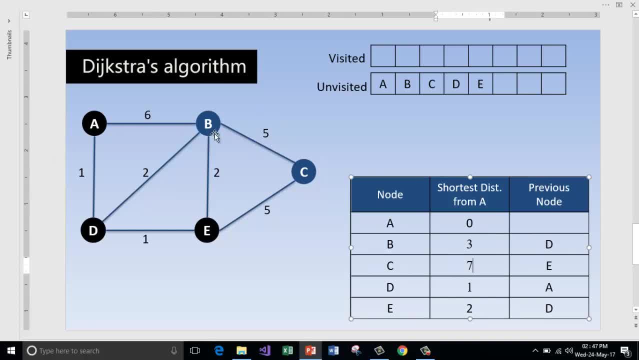 So we are not going to disturb that, But we are marking this as visited And this is the only node that is left in the graph which is not visited. And now we have visited this node, And now we have visited this node And there is no node to visit from this node. 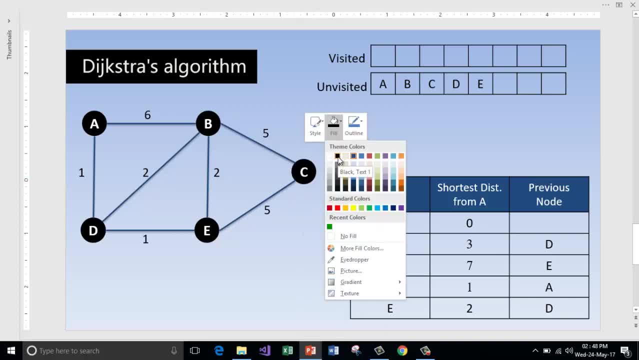 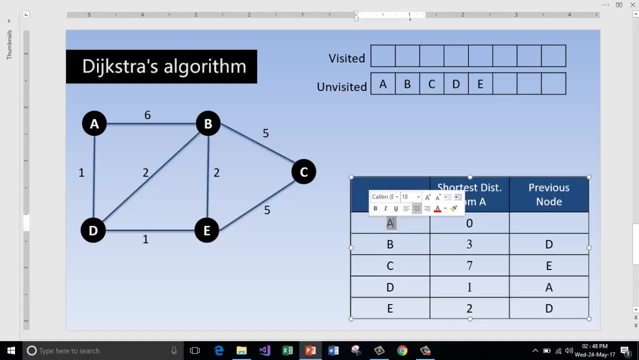 So we will mark this as we did it. So this is also over now. Now look at the table. The cost involved in reaching the node A from itself is 0, and the cost involved in reaching the B from the node A is 3, and so on. 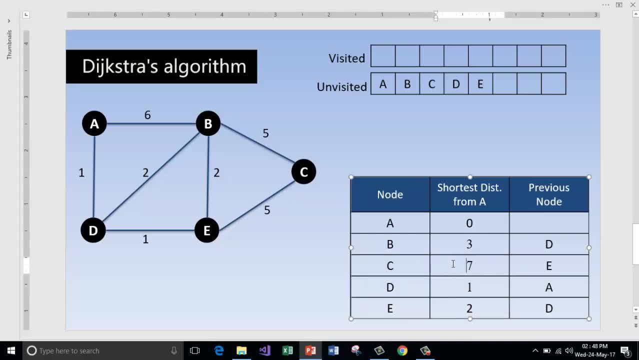 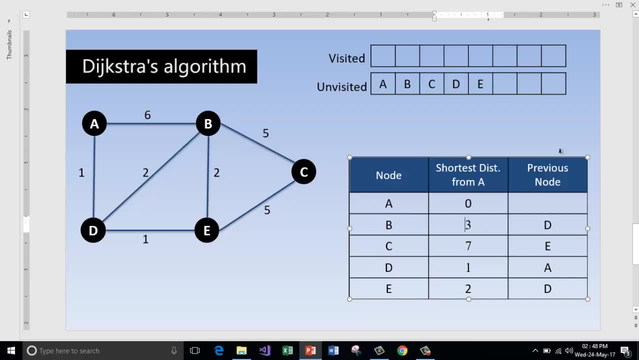 So this is the shortest distance or the shortest path. So this is the shortest path from A to reach these nodes. And here, in this last column, you will find the shortest path. How is that? To reach B, it takes 3 units via D. So to calculate the information about D, go to D. 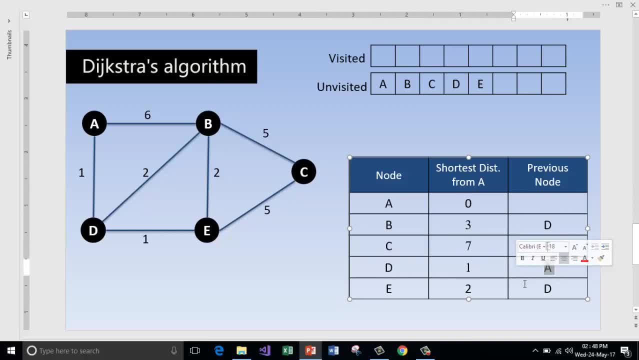 To reach D, it takes 1 unit from A. So that is what we have got: B, D, A is the distance or is the shortest path to reach B, and so on. Okay, I hope you understood this algorithm. If you have got any doubts, please comment below. 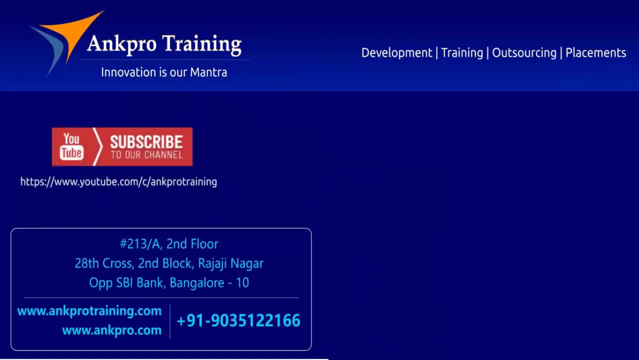 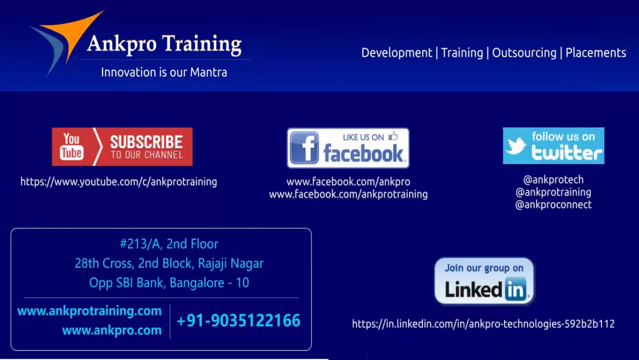 We will try to answer it. Well, friends, that's it for the class. Subscribe to our channel on YouTube, Like our page on Facebook, Follow us on Twitter and join our group on LinkedIn. Thank you.